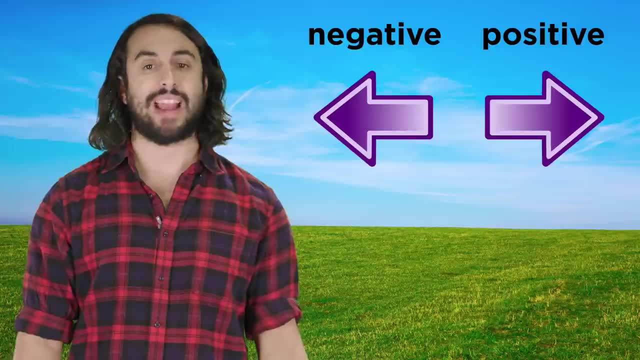 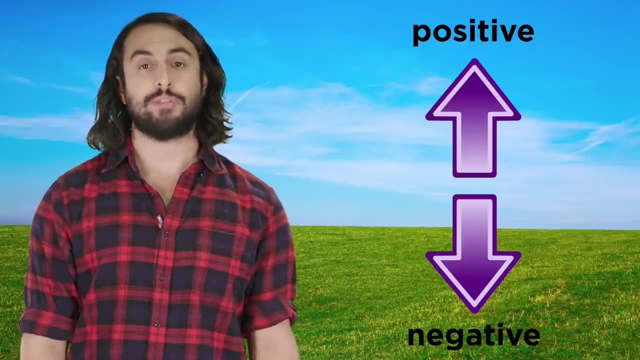 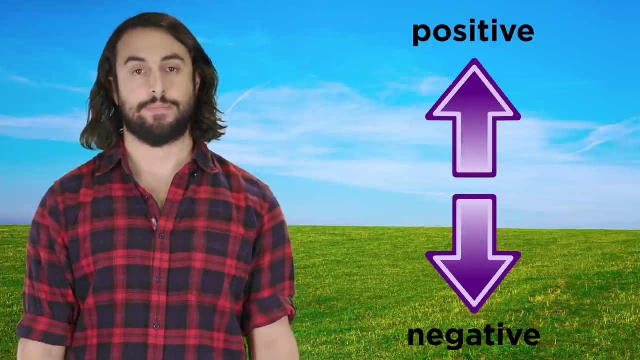 though we often assign the positive direction to the right by convention, But with vertical motion, the negative direction will always be down towards Earth, and objects will always accelerate towards the Earth, since that is the main source of gravity we experience every day. 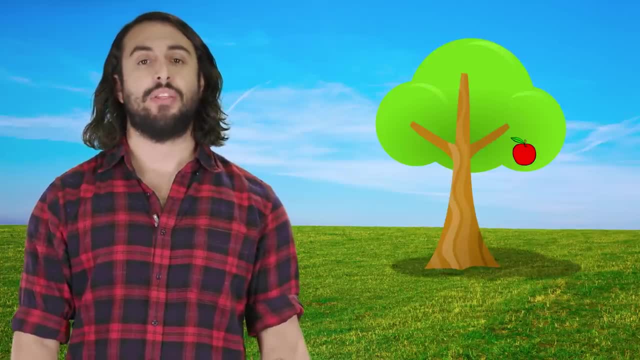 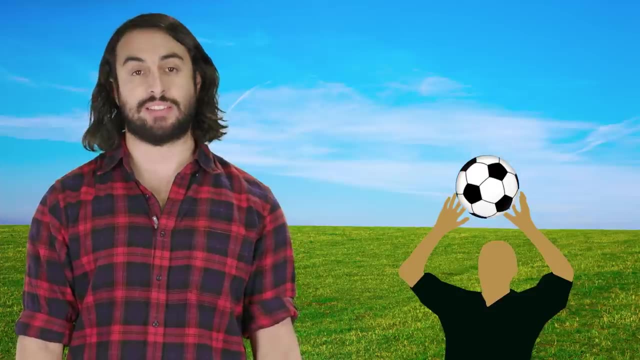 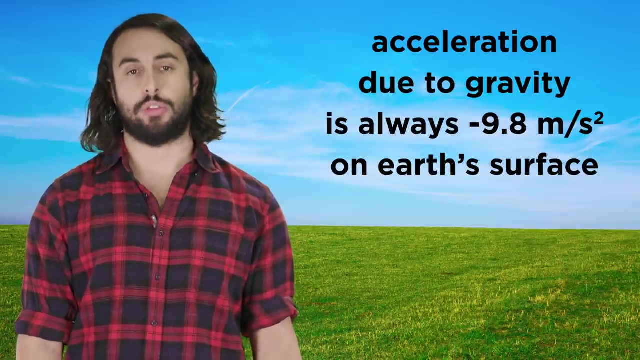 We can examine objects that are in freefall, which means they were dropped downwards from a standstill, or we can look at objects that have some initial upward velocity. Either way, acceleration will always be negative. nine point eight meters per second squared when on Earth, 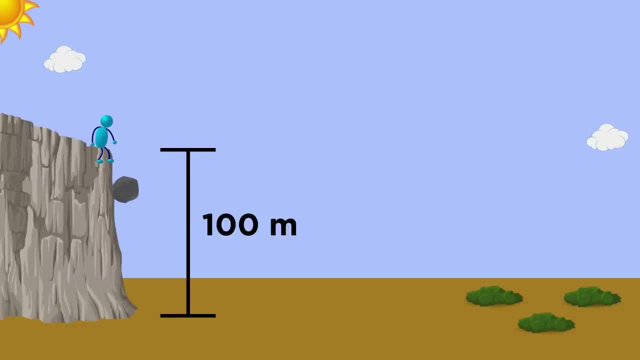 Let's say, for example, you drop a rock off a one hundred meter tall cliff, How long will it take to hit the ground And how fast will it be traveling? To answer this, we will need the equation regarding position, because we know that the 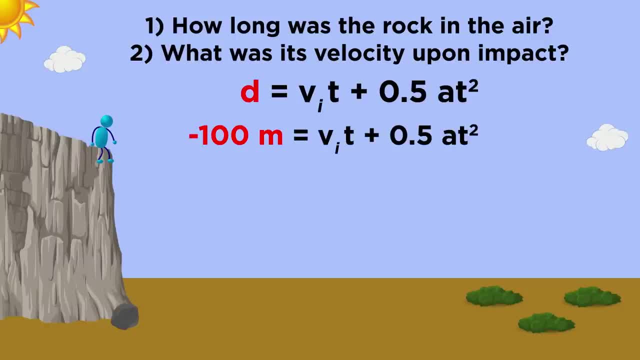 rock must travel one hundred meters in the negative direction. We can plug in negative one hundred here For the initial velocity. that will be zero, because when you drop the rock it is from a complete standstill. Only once you let go does gravity cause the rock to accelerate towards the ground. 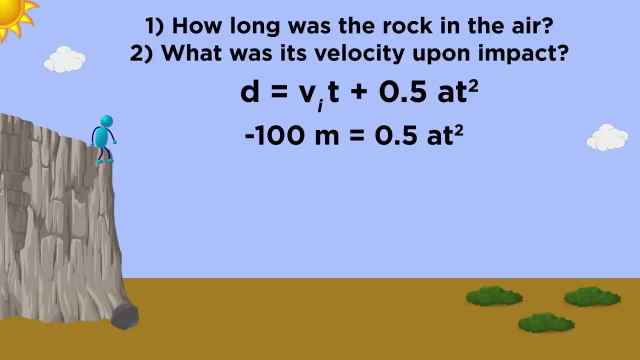 So this whole term can be ignored. Now we plug in the acceleration due to gravity and solve for T. Notice that the negative signs on position and acceleration values will cancel out to give a positive value for time. This is very important as we have to be careful with signs as we do arithmetic, and this will 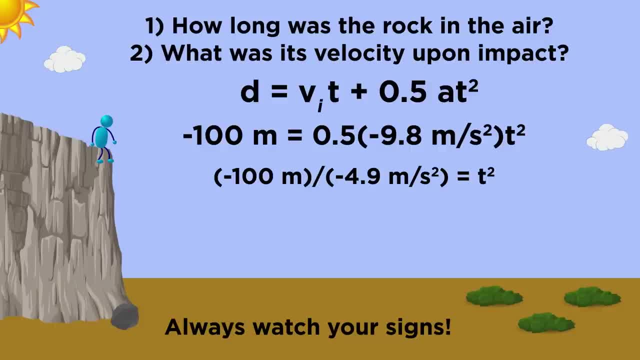 be a common opportunity for error with many students And we get around four point five seconds for the time elapsed during freefall. Now, if we want to know how fast it is going when it hits the ground, let's look at the going when it hits the ground. we can use this equation to solve for velocity. 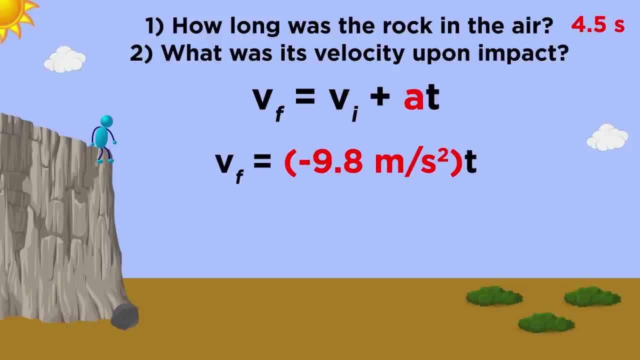 Again, initial velocity is zero and we have negative 9.8 meters per second per second times 4.5 seconds, which gives us negative 44.1 meters per second at the time of impact. This value is negative because velocity is a vector and the object is traveling in the 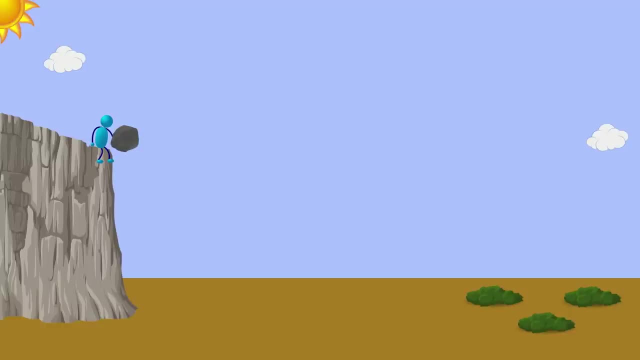 negative direction. Now let's say that we take another rock, and this time we throw the rock straight up in the air with an initial velocity of 10 meters per second. This velocity will immediately begin to decrease because of the negative acceleration due to Earth's gravity. 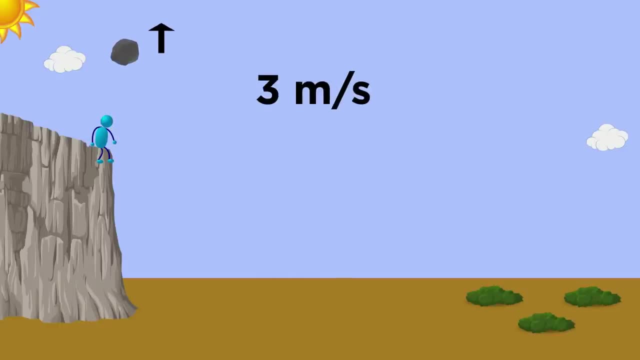 The moment it leaves your hand, the velocity will decrease until it becomes zero and then grows in the negative direction. This means it will travel upwards for some amount of time before falling back down to the bottom where the other rock landed. How long will this rock be traveling before it lands? 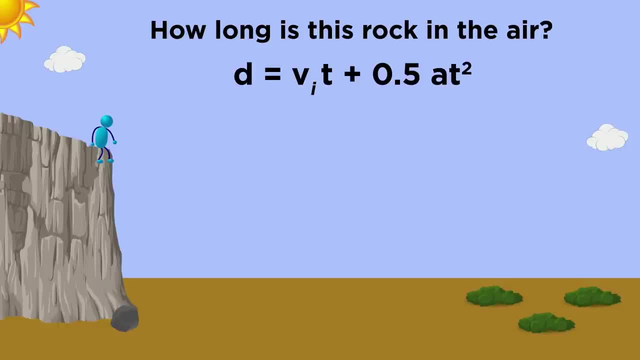 Well, let's do the same calculation that we did before. The only difference here is that, instead of an initial velocity of zero, we have an initial velocity of 10 meters per second in the positive direction or upwards, and the usual acceleration, which again will be downwards and therefore negative. 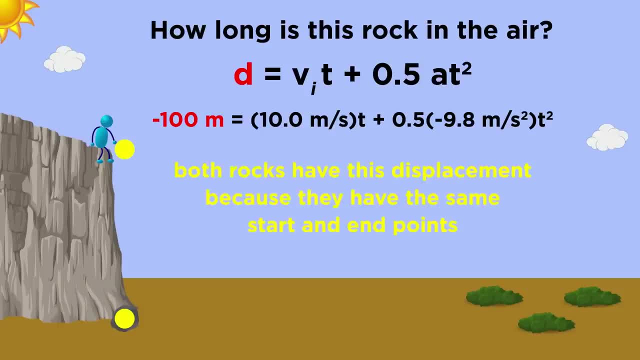 We plug in negative 100 meters for the displacement, remembering that even though the distance this rock will travel is greater than the other one, this rock will keep traveling at the same time one. both rocks start and end in the same place. Then we plug in the other numbers. 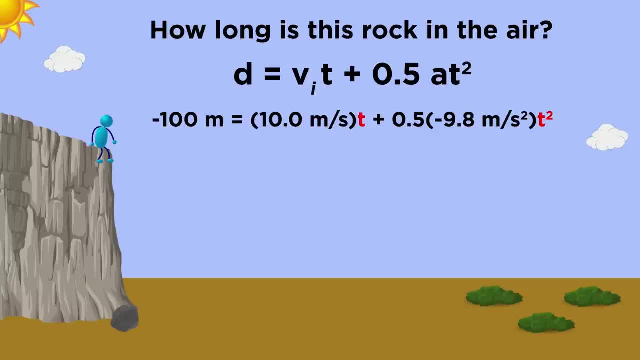 What we are left with is a little trickier than before, because we have both a T and T squared term. This means that we will have to use the quadratic equation. If you have forgotten this from algebra class, here it is as it applies. 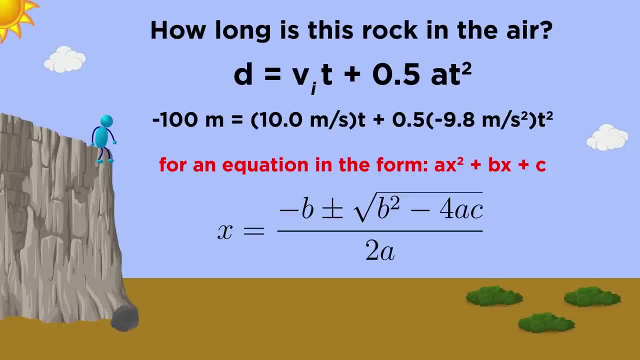 to an equation in ax squared plus bx plus c form. We simply take the coefficients of the equation and plug them into this expression and we will get two answers as possible values for X. So we have to take our equation and rearrange it to look like the standard form, which involves adding 100 to both. 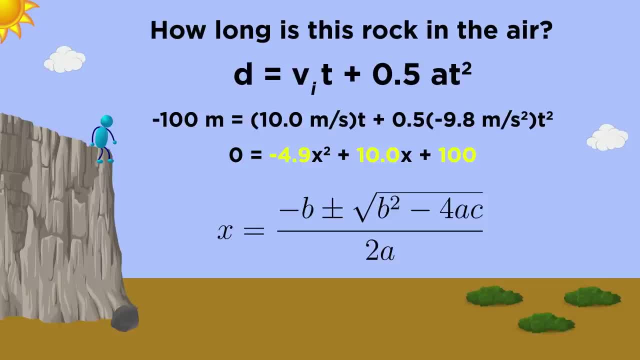 sides. There's our a, b and c. If we plug those in, we get the two values for X, but the positive answer is the one we are looking for, as it doesn't make sense to discuss negative quantities of time. So we can conclude that it takes 5.65. 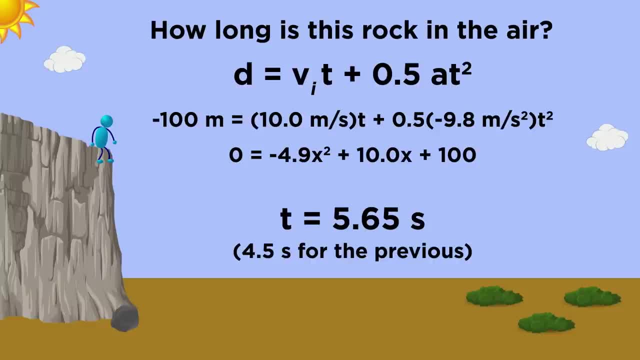 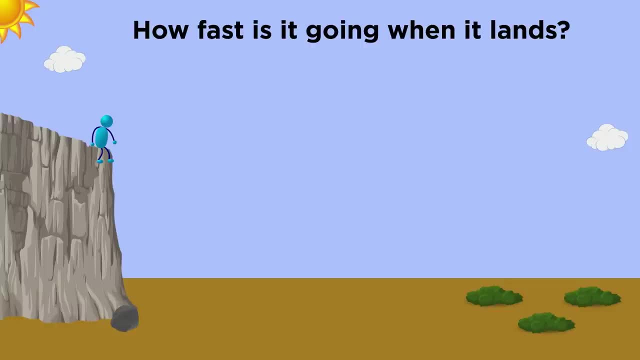 seconds to get to the answer. For this rock to hit the ground a little over a second longer than the one we simply dropped. How fast will this one be traveling at the point of impact? Let's use this equation again. This time we have to use 10 meters per second as the